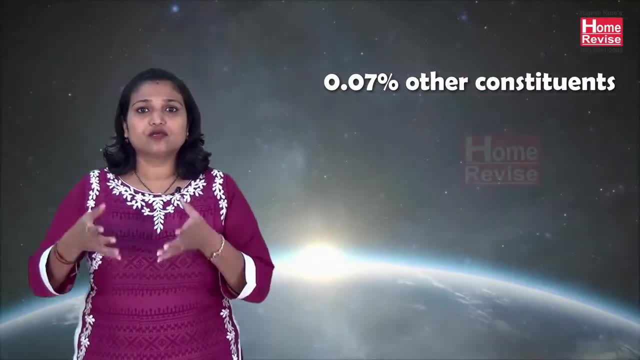 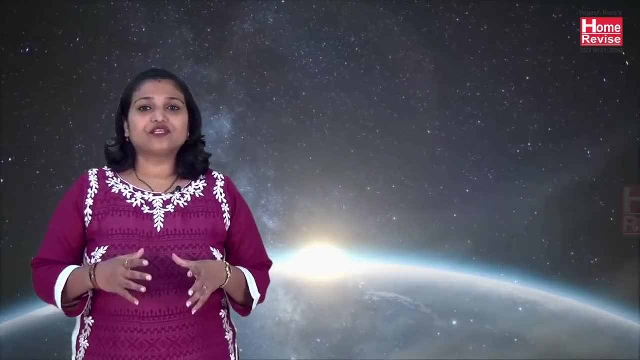 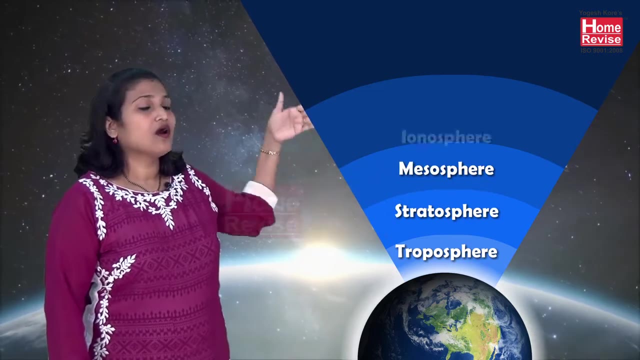 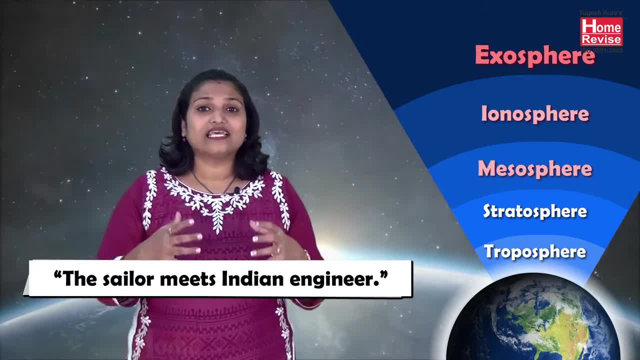 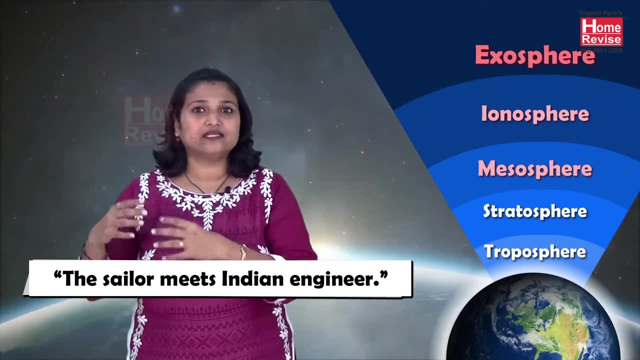 Now further. the atmosphere is divided into five layers: The troposphere, the stratosphere, mesosphere, ionosphere and the exosphere. The sentence goes like this: the sailor meets Indian engineer. I'll just repeat it again: the sailor meets Indian engineer.